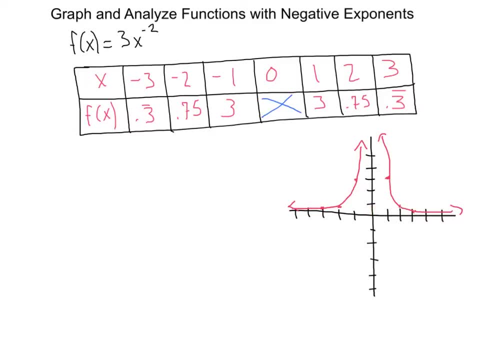 So here we have our graph. Let's go ahead and analyze the components of this graph. Let's go ahead and start with our domain. Here I notice that we have x values for everything except at 0.. x equals 0, we don't have any value. 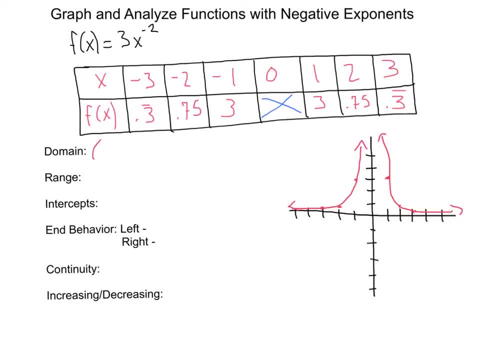 But we do have for everything. So our domain is going to be from negative infinity to 0, union with 0 to positive infinity, Our range here. now we don't have anything at 0 or all these negative values, But we do know that these are getting really, really close to 0. 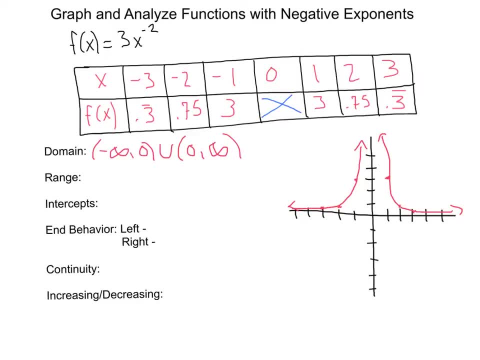 So what we're going to do here for our range is we are going to have a 0, not infinity. So we're going to have 0 included, going all the way to positive infinity Because we have all these positives. But that's why we put a parenthesis here instead of a bracket. 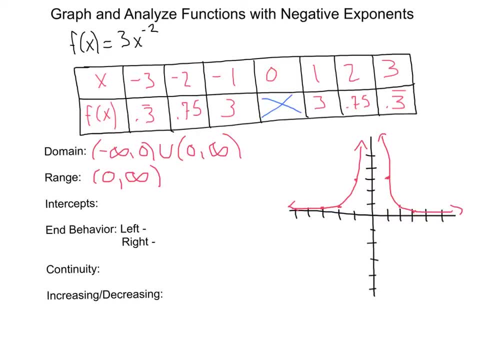 Because this 0 was not included. Now let's go ahead and take a look for any intercepts. I do not see any intercepts here on the graph. I look here at 0, where you might think where intercepts have typically been. 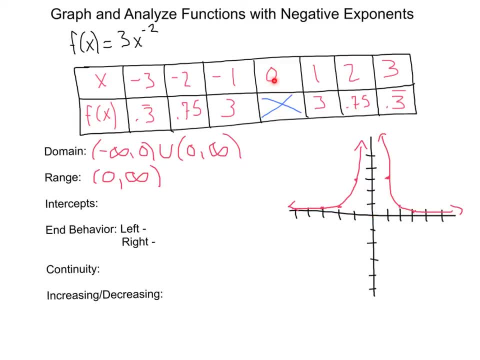 And our value is undefined Because, remember, we can't have a 0 in the denominator And when we rewrote this as 3 over x squared, we can't have a 0 down there, So we don't have a value. 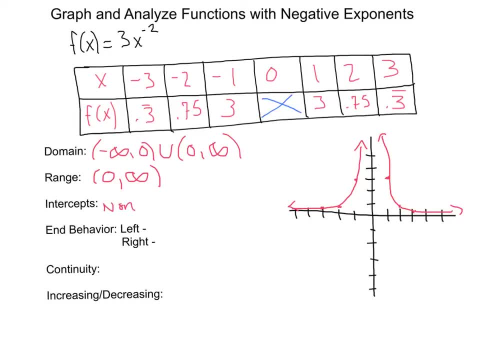 We have no intercepts. So intercepts, we have none. Our end behavior: as we go to the left, it looks like it's getting closer and closer to 0.. As we go to the right also, we are getting very, very close to 0. 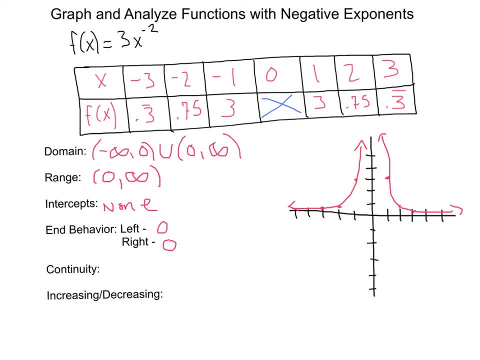 Now let's look at our, Our continuity. here We're continuous all the way until this break. right here We have a gap. right here, at x equals 0.. So what we can say is we are discontinuous: at x equals 0.